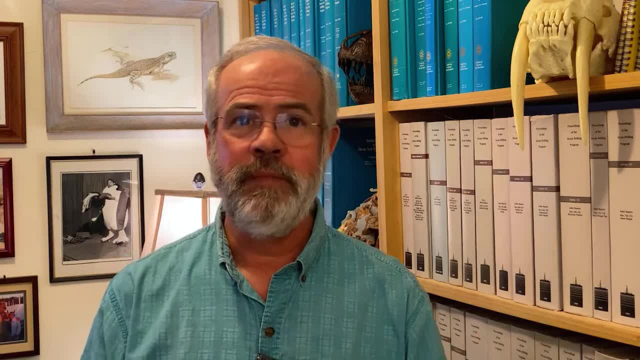 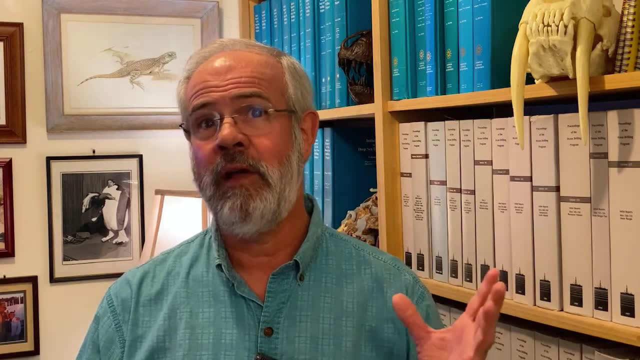 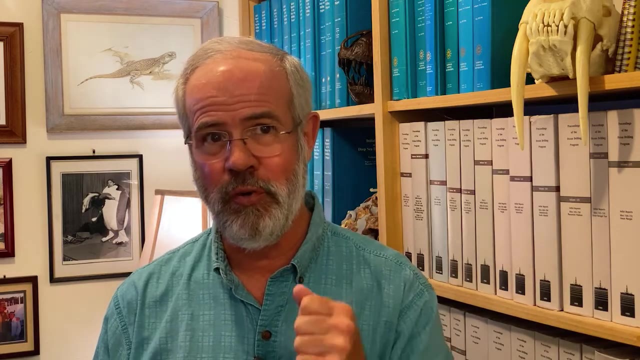 has done to Earth and how Earth's evolution has affected life. There's a lot of detective work in paleontology and we will show you how the pieces fit together and also where we have big questions that remain. I love this stuff and will try to convey some of that excitement to you, So enjoy. By the way, we 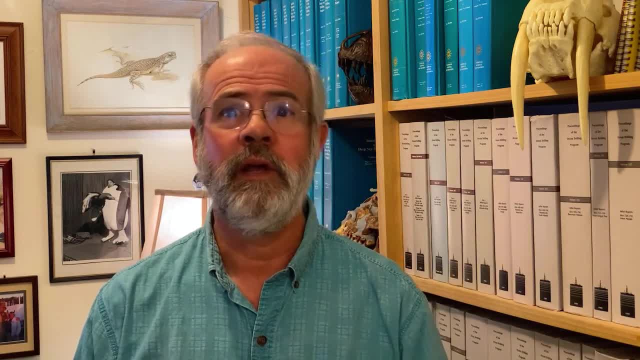 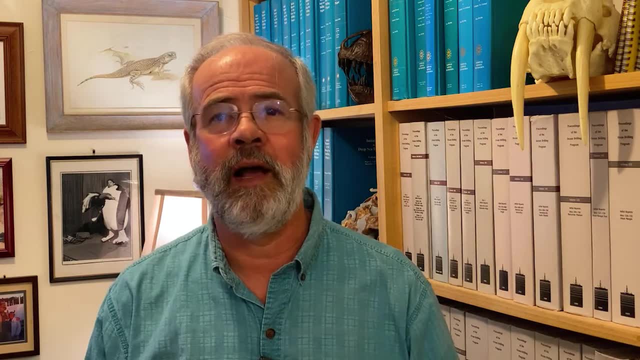 have three books for the class that I use in my university course that are for supplementary reading. All are pretty cheap, namely 10 to 15 bucks, and they cover different parts of the class. Life on a Young Planet by Andy Noll covers. 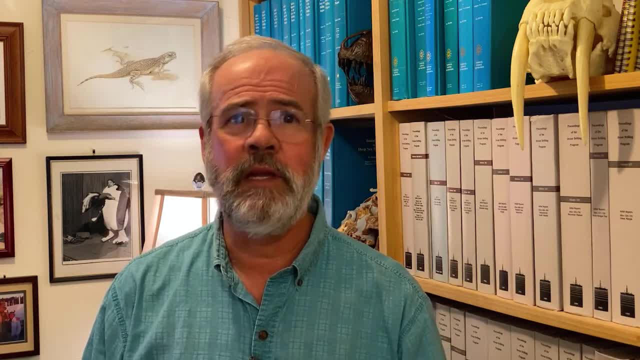 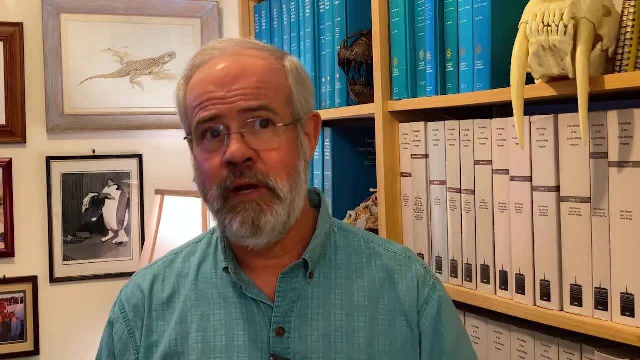 the first third of the class Noll addresses the first four billion years of Earth history, from the dawn of microbial diversity to the appearance of animals. Your Inner Fish by Neil Shubin covers the next third. Shubin does a great job showing where 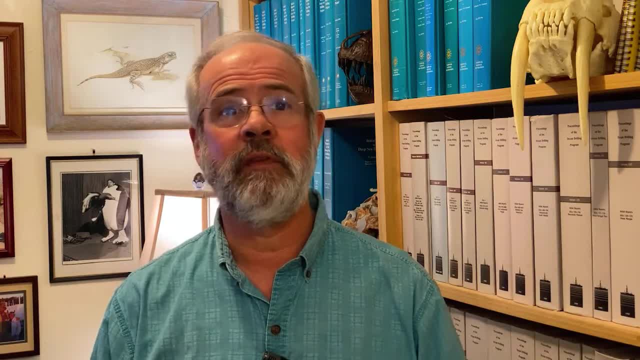 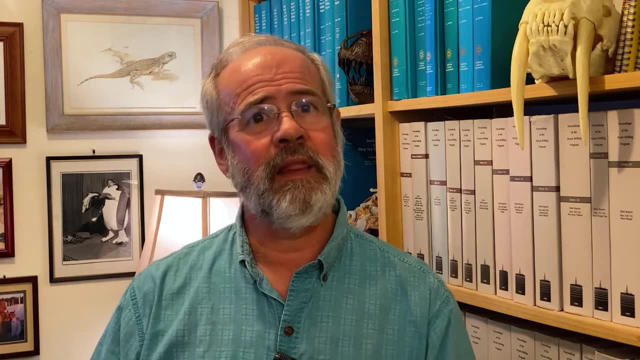 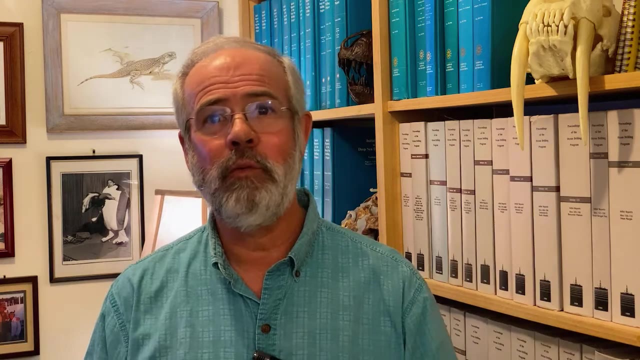 vertebrates come from. He also participated in a lovely BBC production, also called Your Inner Fish. The Earth After Us covers parts of both the beginning and the end of the class and addresses what the paleontological record of our time might look like, What would be recognizable and what would. 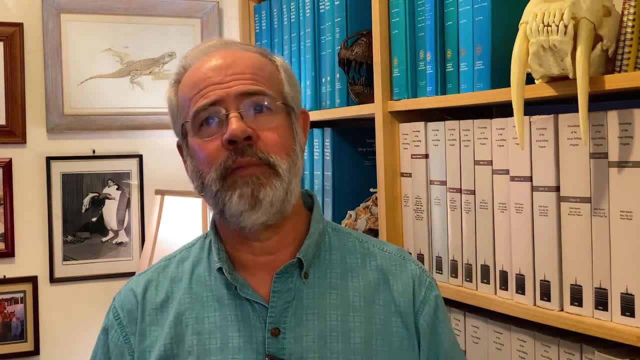 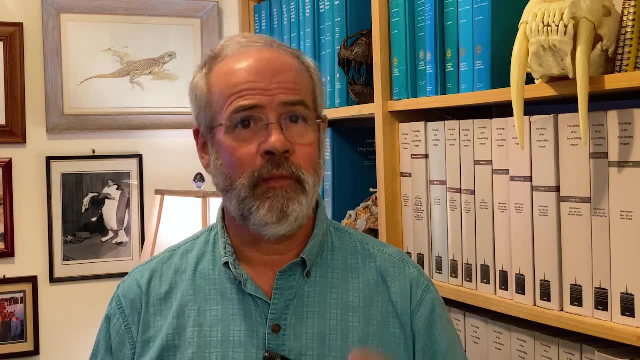 vanish with the ages. There are also a lot of new books appearing every day, reflecting the rapid pace of discovery in paleontology. I'll mention those as we go along. So with that, here we go. 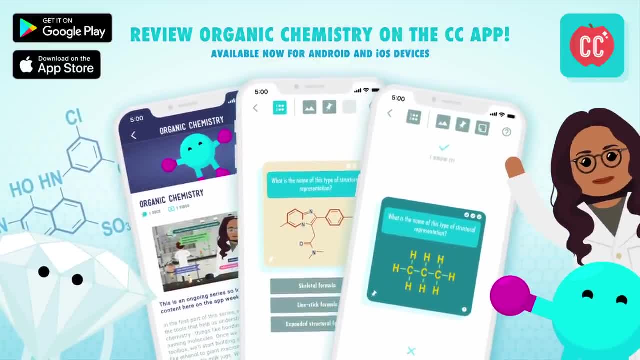 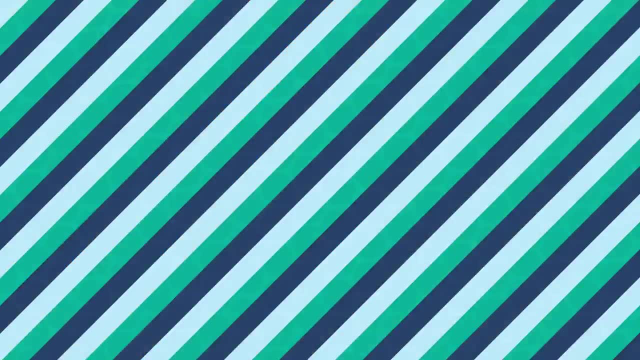 You can review content from Crash Course Organic Chemistry with the Crash Course app, available now for Android and iOS devices. Hi, I'm Deboki Chakravarti and welcome to Crash Course Organic Chemistry. The Australian Blue Mountains and the American Blue Ridge Mountains both get. 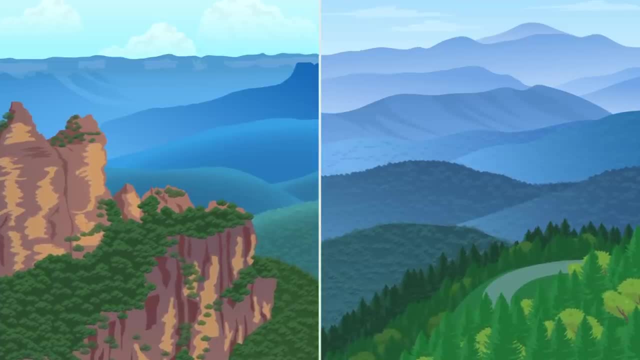 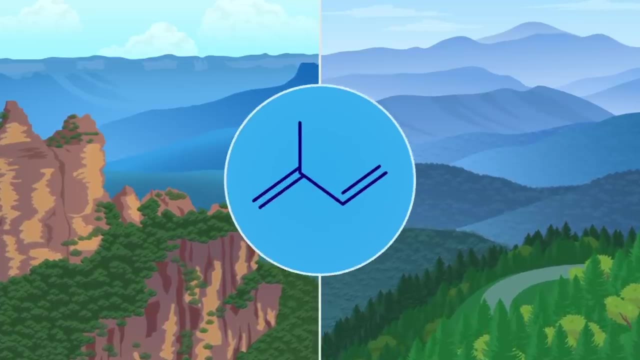 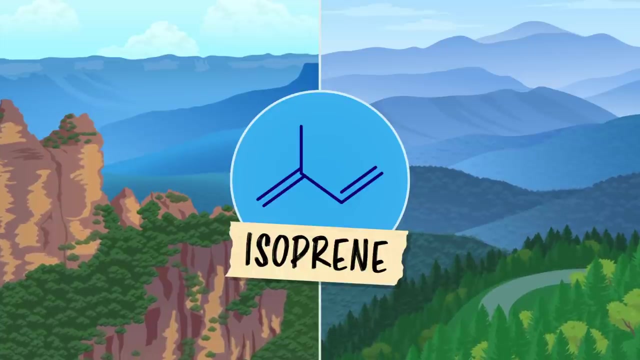 their colorful names from a blue haze that blankets them on hot summer days. This haze comes from small molecules that scatter sunlight, specifically small wavelength blue light. One of these small molecules is isoprene, a volatile, biogenic organic compound, or, in simpler terms, an organic chemical made by living things.